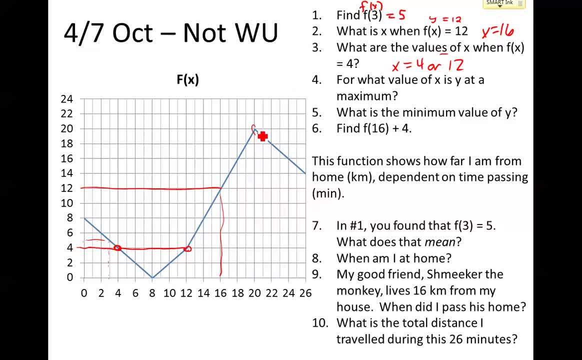 So we look for the maximum y, which is right there, And it asks: what is the value of x when y is at a maximum? And so the answer would be 20.. x equals 20.. Now what is the maximum value of y? 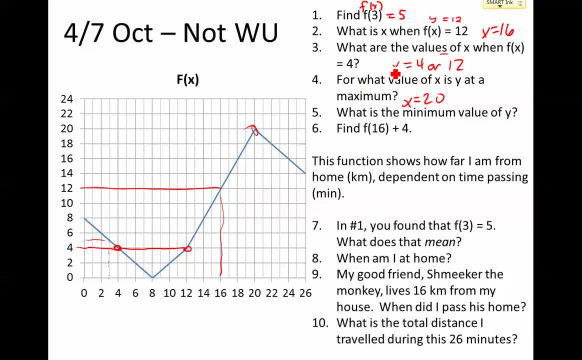 Well, that's also 20.. But this question is asking for what value of x is y at a maximum? So it will be this: 20.. All right, what is the minimum value? So f of y? we go to the lowest point, and the minimum value of y is, of course, 0.. 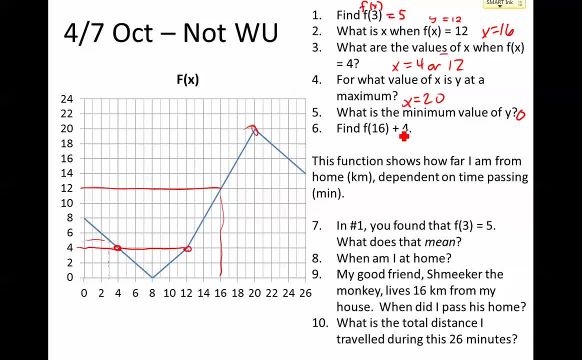 Very nice- And find f of 16 plus 4.. So again f of 16.. So f of x. So the x has been replaced by 16.. So first we need to find the f of 16, because this should happen before the addition. 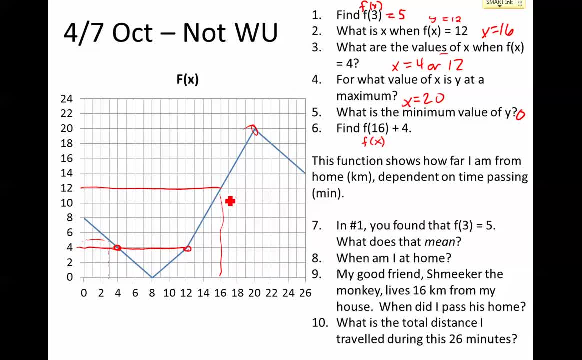 So we'll go to x 16, which is right here, And we find out that that is 12. So f of 16 is 12. And then we'll add 4, which is a total of 16.. All right, now, it gives us a little bit more information. 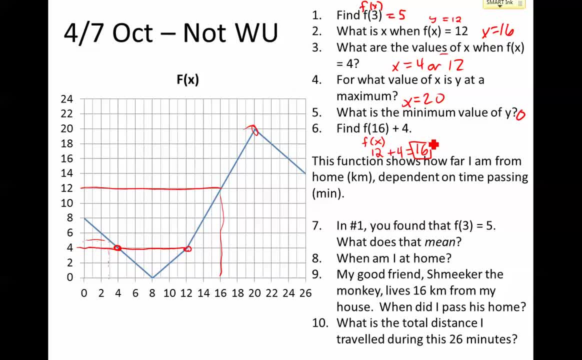 It says, this function shows how far I am from home in kilometers, dependent on time passing. All right. so this tells us a couple of things. Number one: it tells us what exactly is being related here, But it also tells us what's on the x-axis and what's on the y-axis. 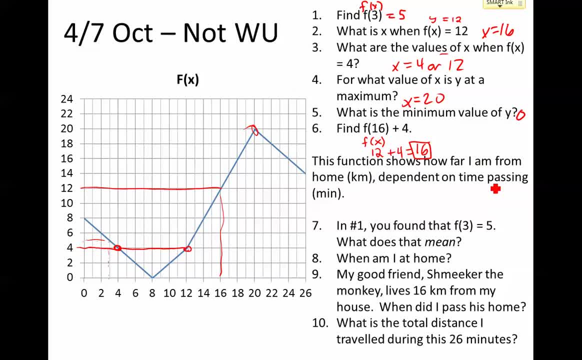 It says how far I am from home is dependent on time, And so how far I am is the dependent variable which always goes on the y-axis. So this is how far from home, of course in km, All right, and then the x-axis. here is time in minutes. 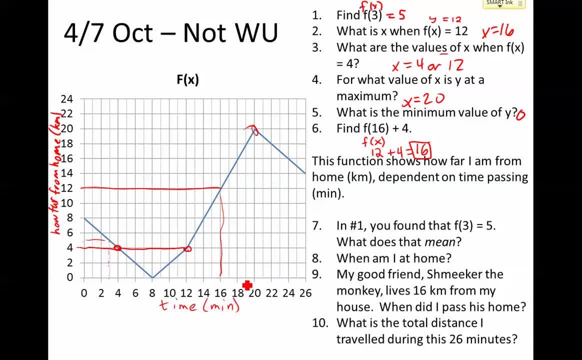 Very good, very good. So, number seven. In number one, you found that f of 3 equals 5.. What does that mean? Well? what does that mean? Well, the x has been replaced by 3, and x is the time. 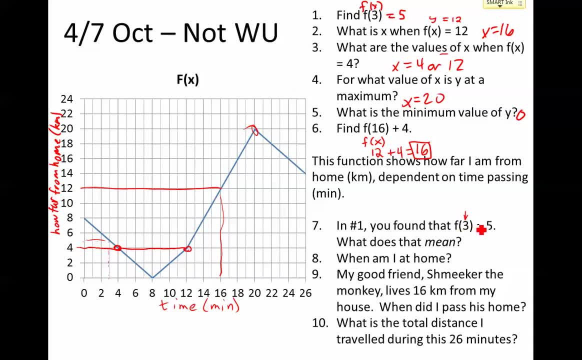 So when the time is 3 minutes, the result or the output is 5, which is the distance from home. So after 3 minutes I am 5 km from home. That's what this statement means. It's a very simple statement. 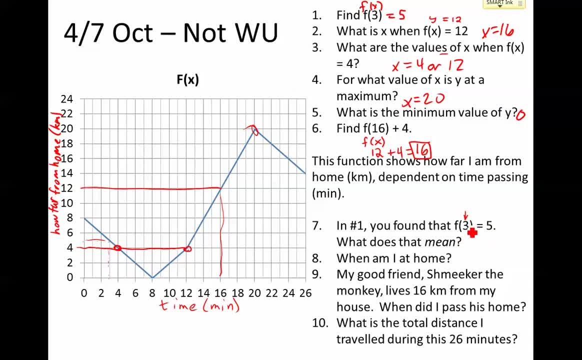 Yet from that I can see that the x value of the time is 3. And the y value- the distance from home- is 5.. When am I at home? Well, when I'm at home, how far am I from home? 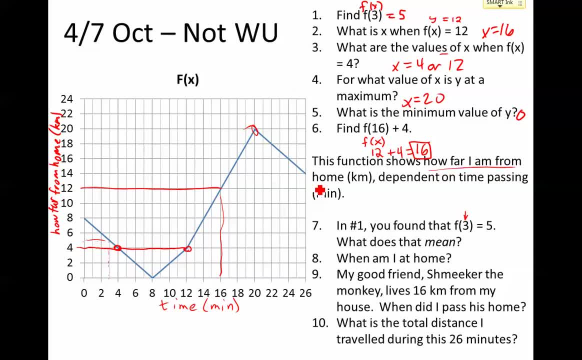 Zero. So I want, how far I am from home, the distance to be zero. So we go to where the distance is zero And right here we see that that is at 8 minutes. All right, My good friend Shmiko the monkey lives 16 km from my house. 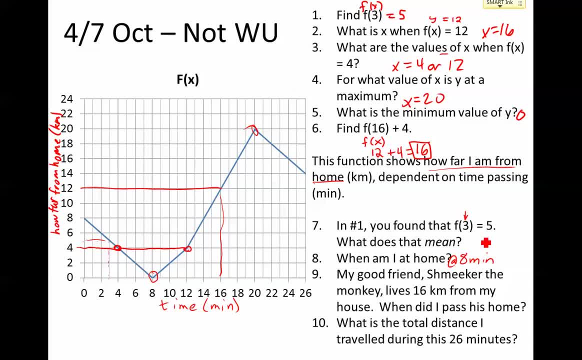 When did I pass his home? All right, So 16 km from my house. So I'll go up to how far from home 16. And I'll go over here, Whoop, Whoop. So I actually passed Shmiko's house twice. 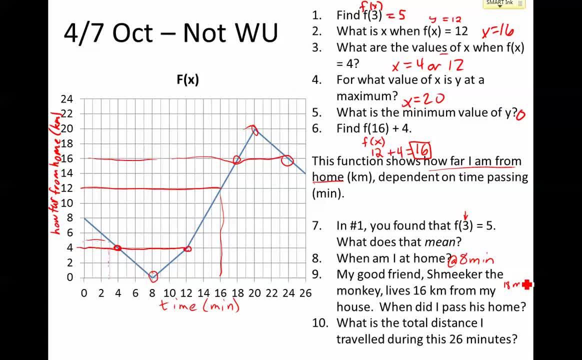 One of them is at 18 minutes And the other one is right here at 24 minutes. Sweet Last. what is the total distance I traveled during this 26 minutes? Well, this is distance, So I need to count up all the distances I traveled. 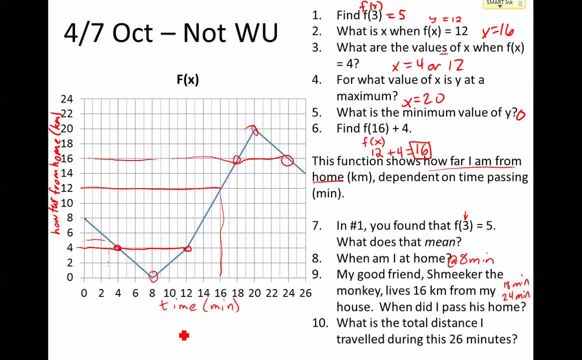 So from here to there I traveled 8 km because I went from 8 away to 0 away And then I start going away from home and I travel up to 20. So I need to add on a 20 there. 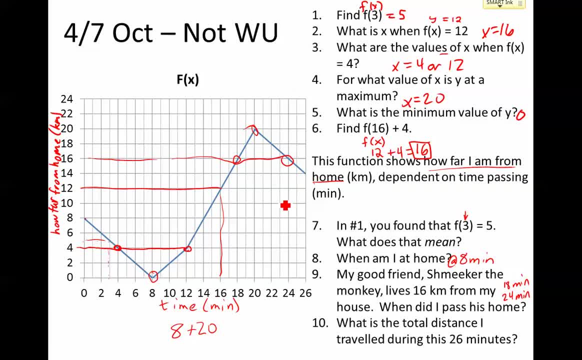 Okay, And then from 20, I come back to 14. So that's another 6.. So I should add all those together: 8 plus 20 is 28,. plus 6 is 34 km is my total distance. 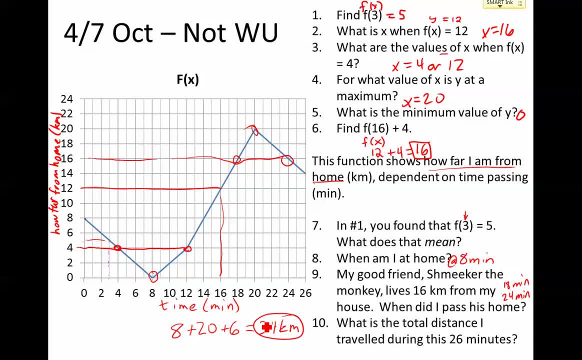 All right. So hopefully you got those questions right. They weren't too bad, But yeah, do those in about 4 or 5 minutes. I did them pretty quickly and I'm talking through every single little detail. All right, So see you in class.